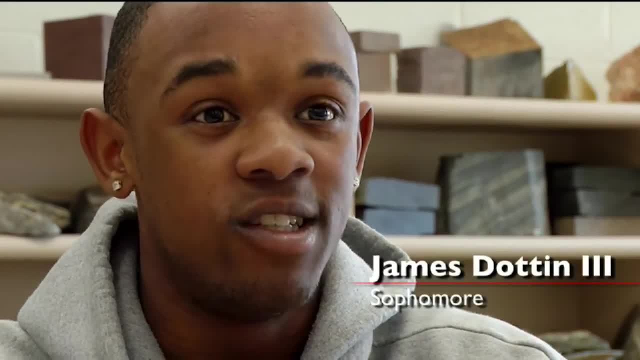 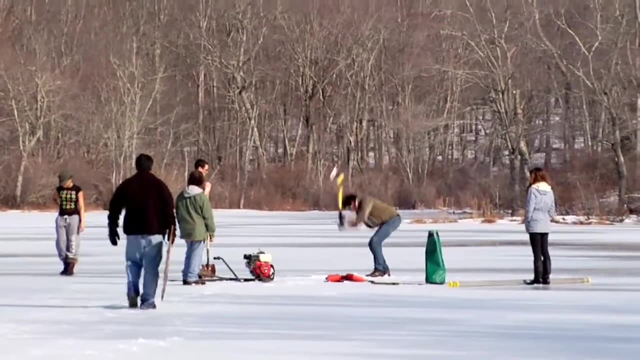 When we were out in the field, it was good to see how to actually take these different types of cores using different equipment. you know, learning how to gauge, like if you can walk on the ice, you know, in order to take an ice core from a pond. 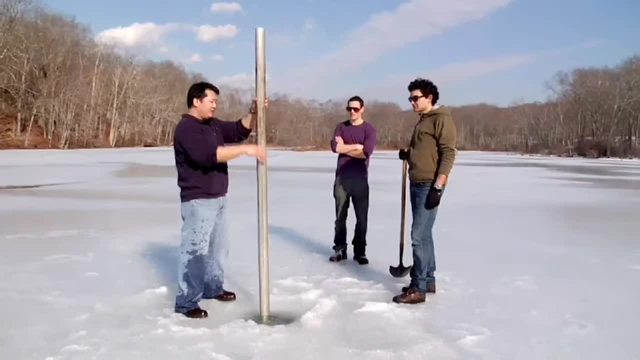 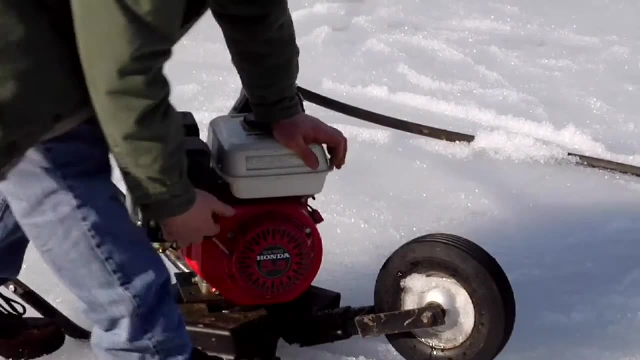 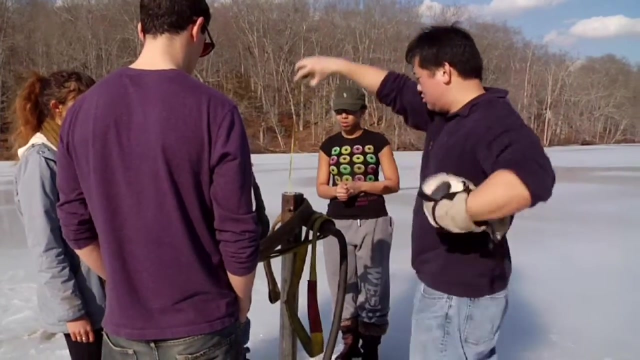 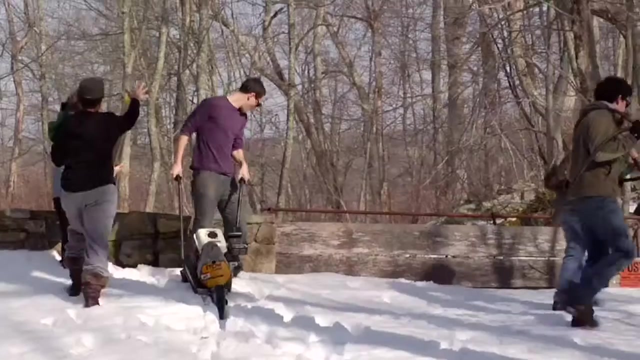 This is a lot of wood, just like anything else. We had to draw a map and mark where we were taking our cores from, and then we hauled everything back to the vans and brought it all back here, And then so we'd lay out the cores on the tank. 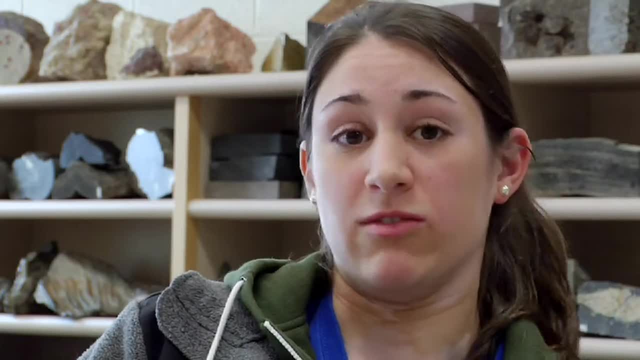 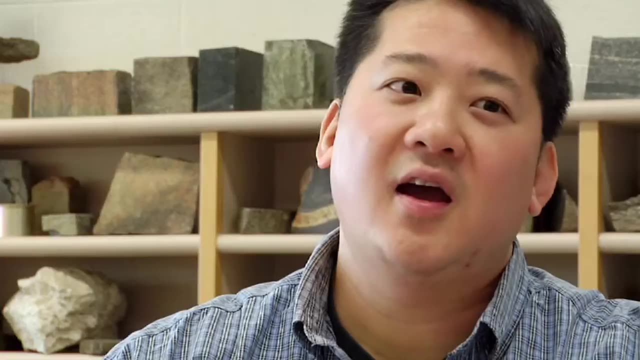 Yeah, and we take out samples for every five centimeters or so through the depth of the core. The students are looking at the sediments behind where the dam was, and they're looking mainly at two things. One: is there a release of nutrients or metals? 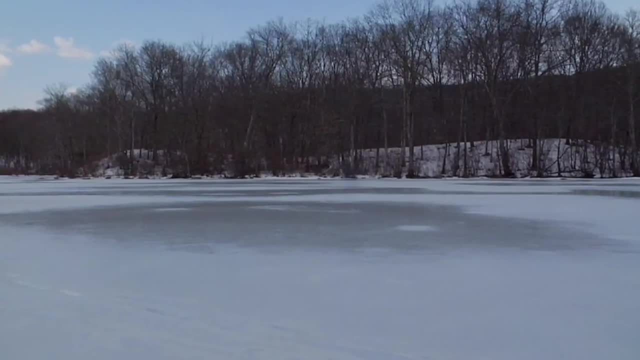 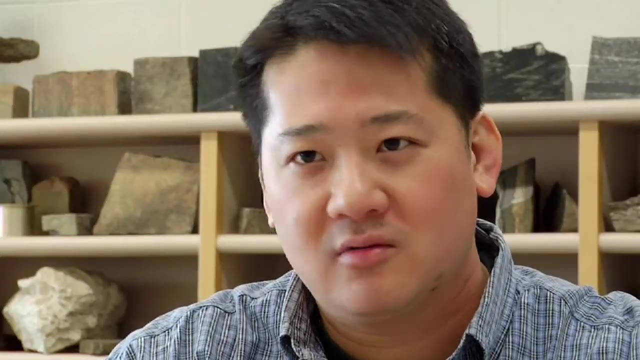 And the other aspect is: can we use those sediments as an archive? So the idea is that we can go back in time and figure out what was going on at that site before the dam was put in, while the dam was there for 100 years or so. 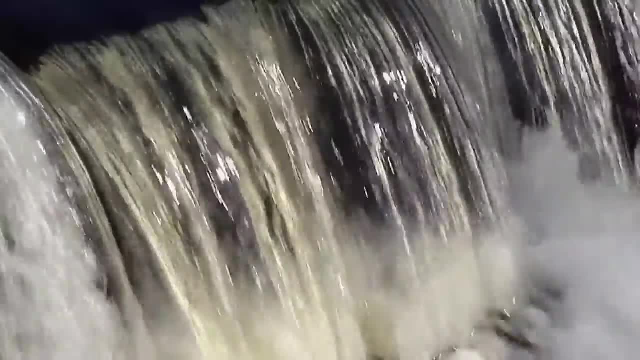 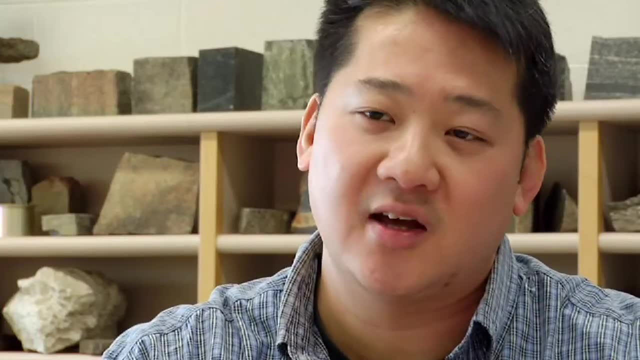 and then after the dam was removed. If you removed the dam and they did it improperly, there would be a flood of sediments coming downstream. So we're trying to see if there was a change in the sedimentation at that site. My part of the project is to measure the phosphorus sediment. 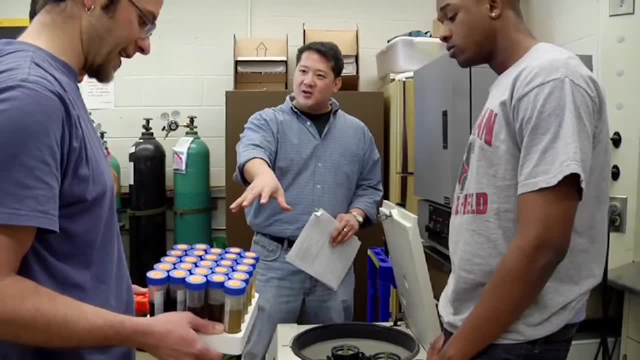 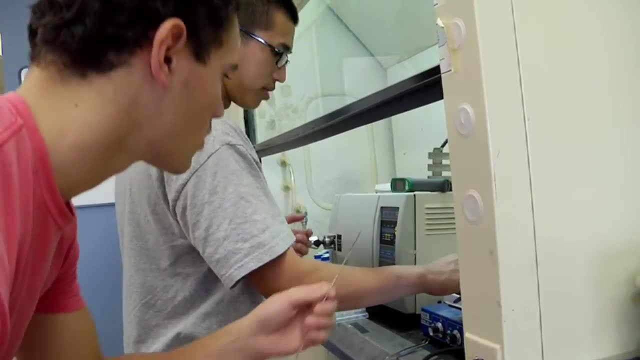 from the ice cores and the fiber cores that we took. We are trying to find out how much biogenic silica is in it, trying to see if there's still the same level of silica as another part of the river where there wasn't a dam. 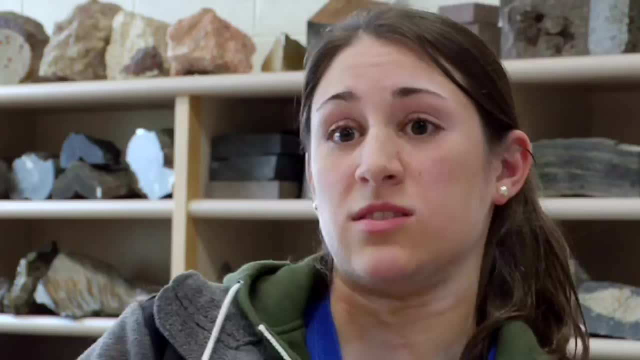 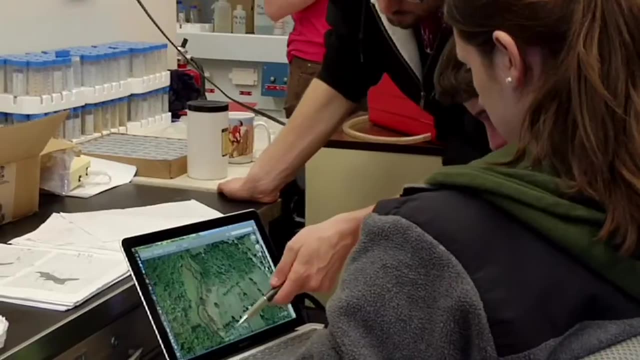 We're doing mercury analysis on each of the individual sediments to see how mercury concentrations in the marsh have changed over time. My group is also looking at stratigraphic sections, So we have drawn diagrams of all the cores. We have pictures of all the cores in segments that we've just stitched together in Photoshop. 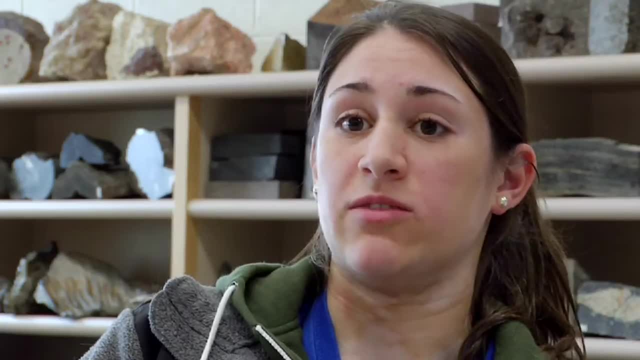 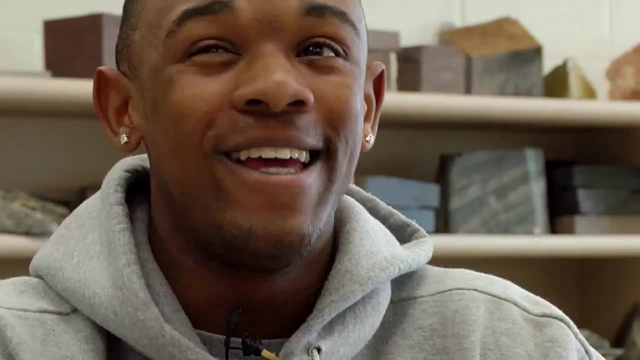 so that we can see the variation through the depth at different places within the marsh, And we'll try to come up with some sort of a story on how all that happened. Here we get to use the centrifuge, We get to use the different equipment. 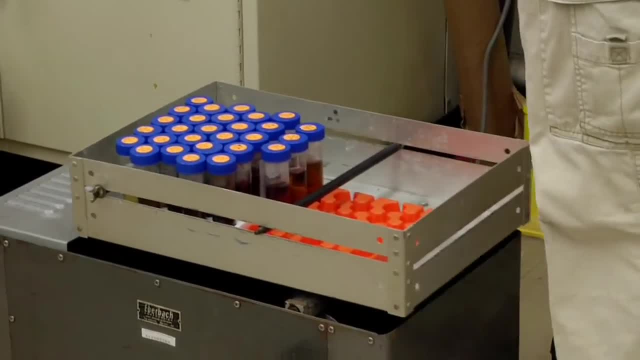 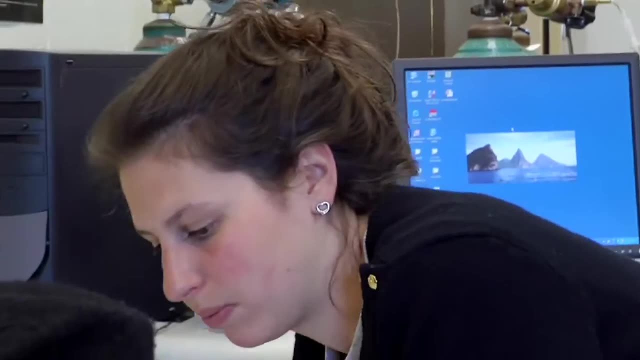 And I feel like I'm getting the opportunity to learn. It's a lot more exciting than me having to go through a procedure and then write up about it, even though a lot of people have already done it, and nobody's done what we're doing today. 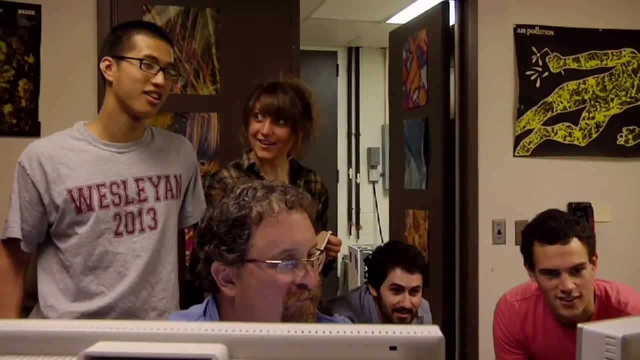 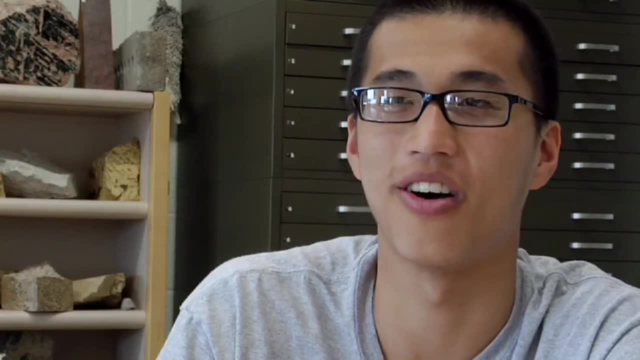 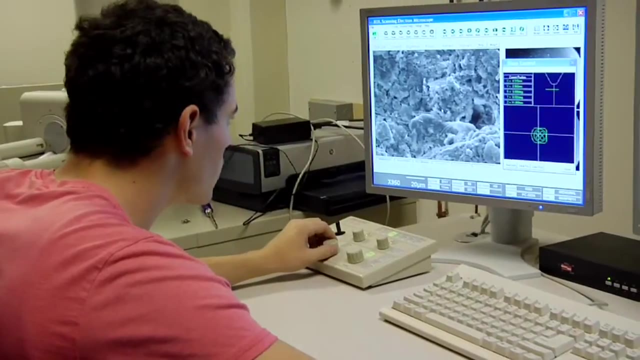 Oh my god, Awesome. That's so cool. We're actually getting our own materials and then we have all this equipment. that's different and everyone's doing something different. We're doing microanalysis- The majority of our experience with the project. 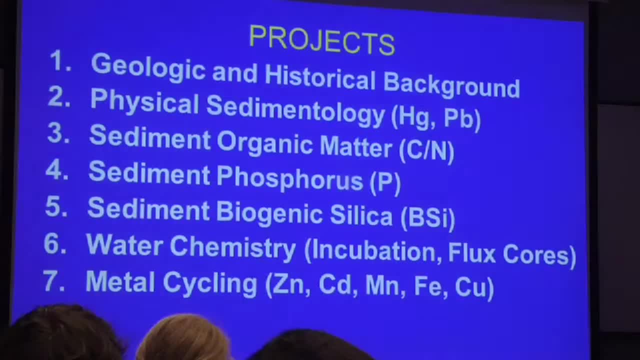 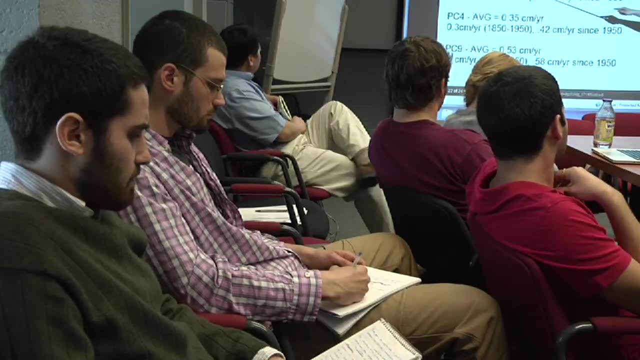 will actually be in a couple weeks when we give our final presentation. Connecticut currently has more dams per mile of waterway than any other state in the United States. To combat these anthropogenic effects, Nature Conservancy has designated 21 sites as preservatives of these wildlife areas. 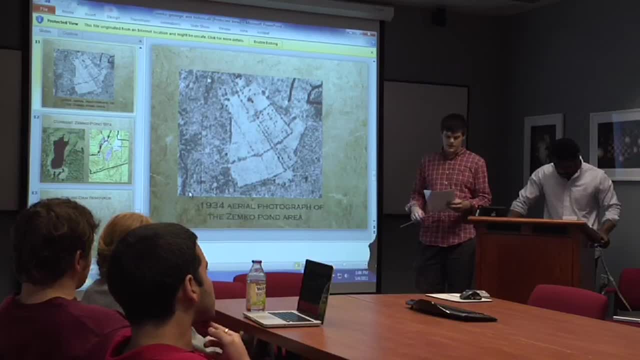 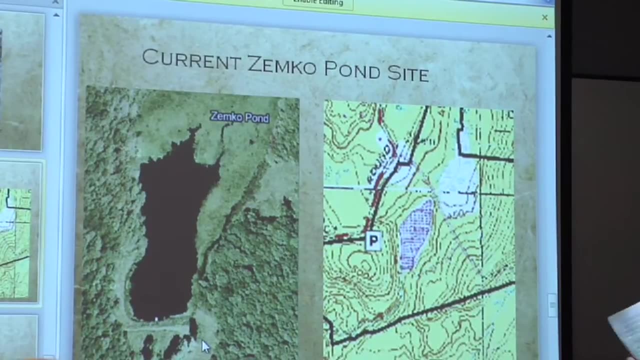 The Zumco Dam that we studied in particular is a privately owned structure recently purchased by the Nature Conservancy. Now that the dam is gone, studies like ours focus on the geologic changes that, in turn, affect flora and fauna, ecosystems and help provide a better understanding of river recovery. 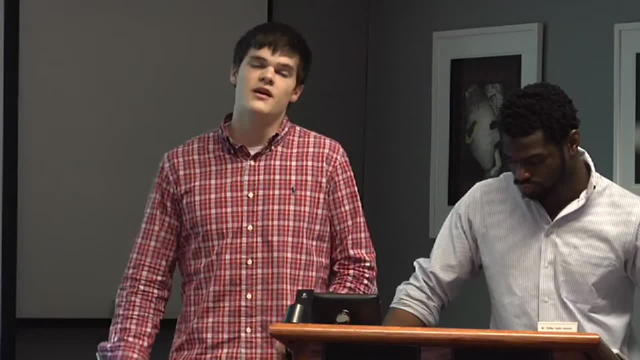 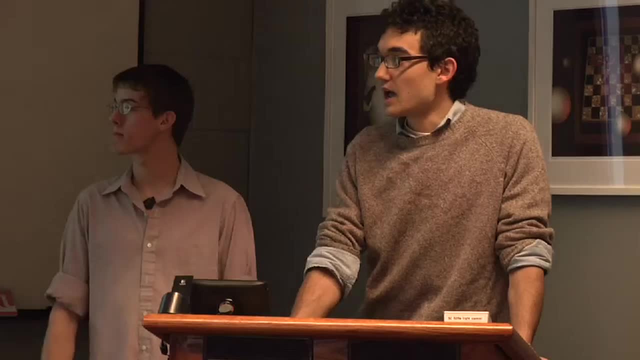 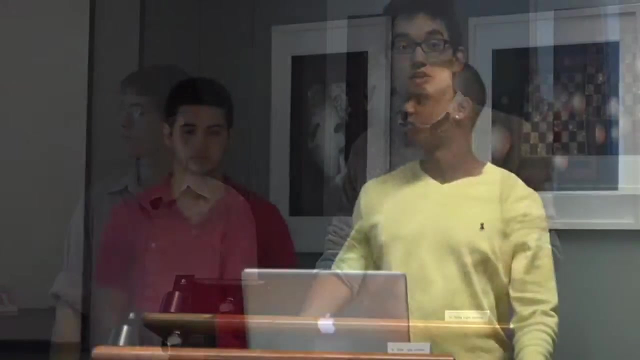 after dam removal, guiding future restoration projects around the Northeast and the entire world. For our study, to study the sediment of the area, we took peat cores and from these cores we were able to analyze the mercury and lead concentrations. Phosphorus is an essential element in biological activity. 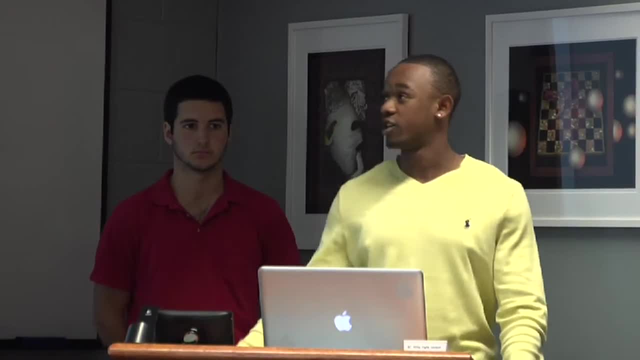 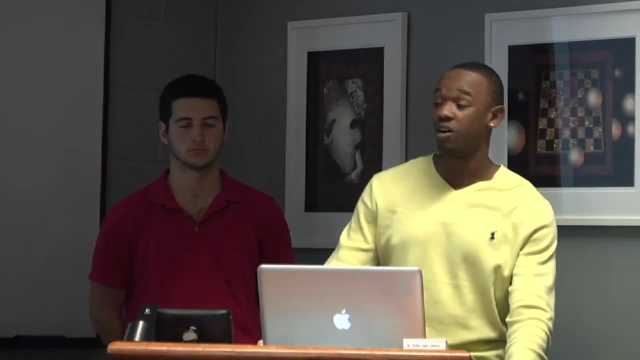 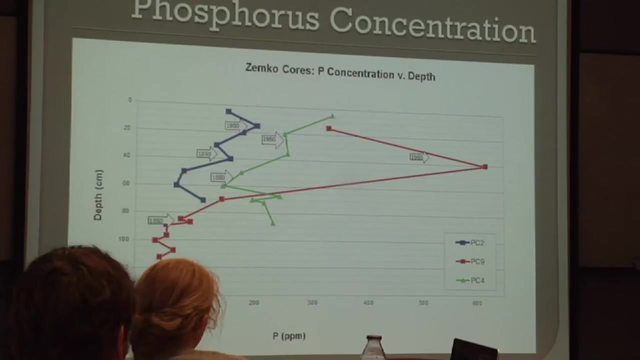 Such as sustaining the life of plants and other terrestrial species. Its relative concentrations can tell us the source of organic matter that would have metabolized the phosphorus, And understanding of this element in samples allows us to determine environmental conditions in the water, such as oxidation reduction. state of the water. 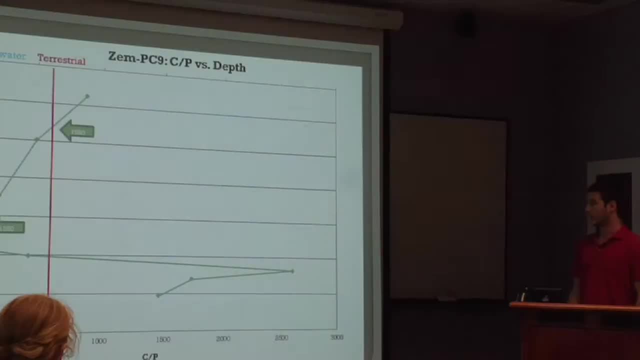 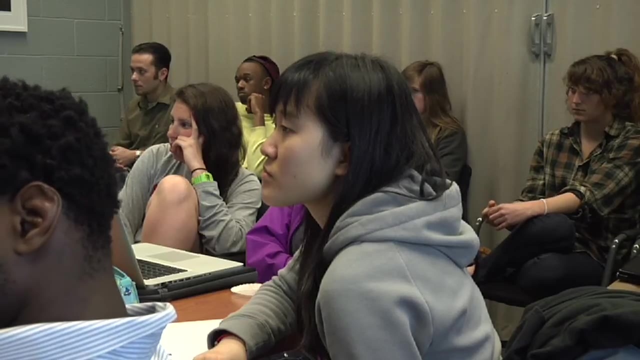 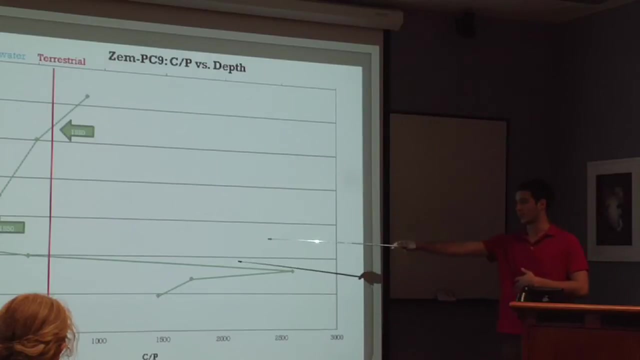 biota identity and trophic state. In the last peat core we see something more interesting sort of happening where in the far past there was a much higher ratio of carbon to phosphorus And then somewhere around this time period there was something that caused a rapid decrease.